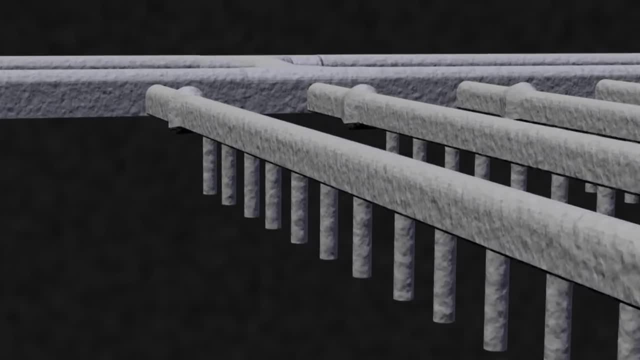 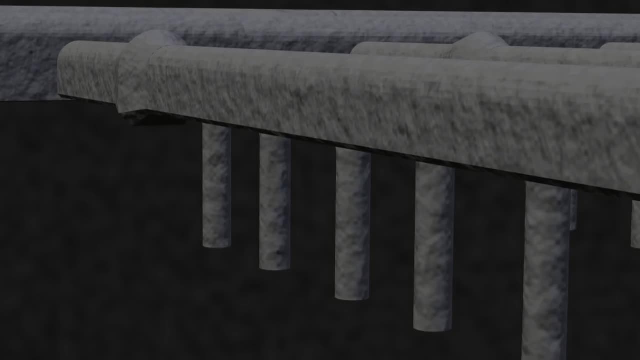 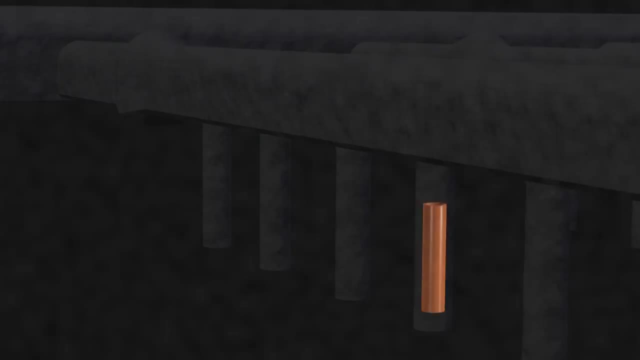 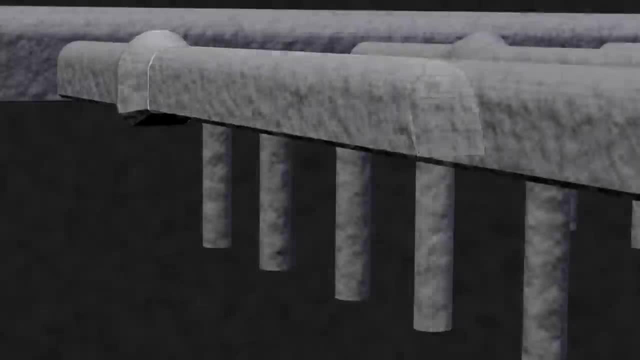 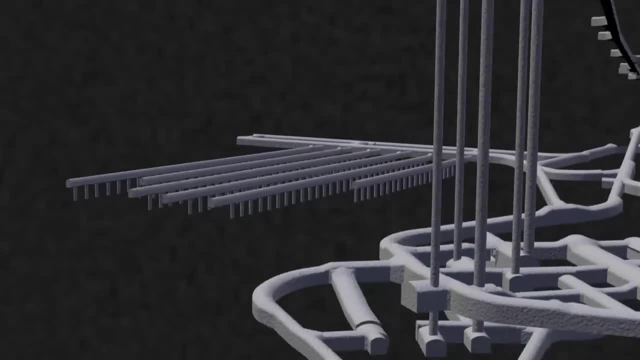 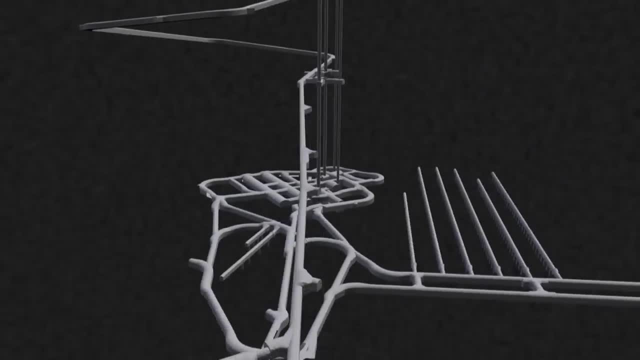 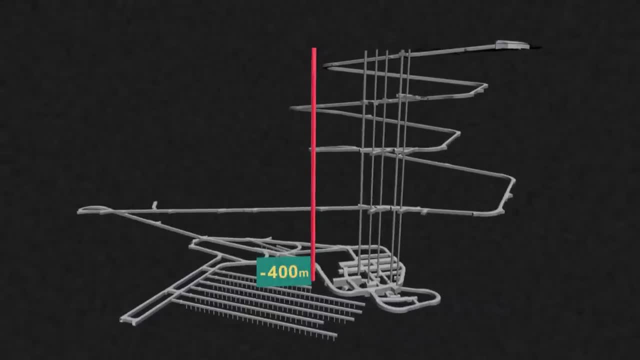 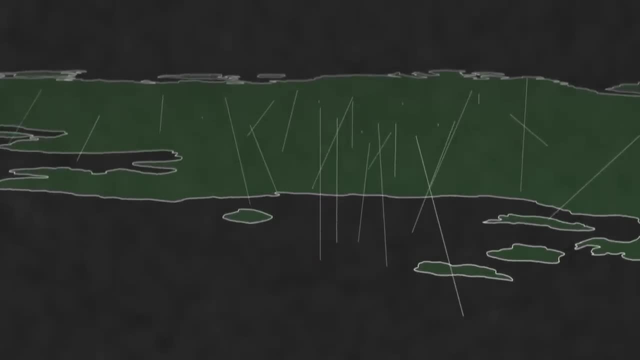 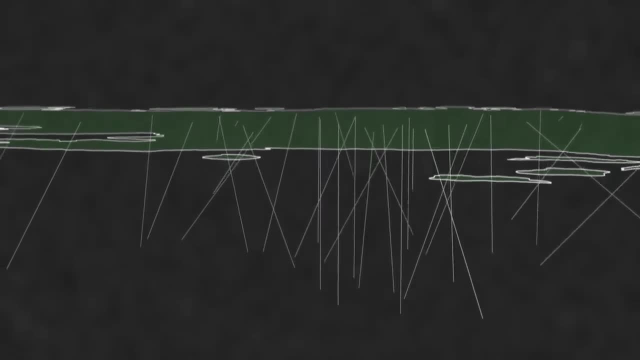 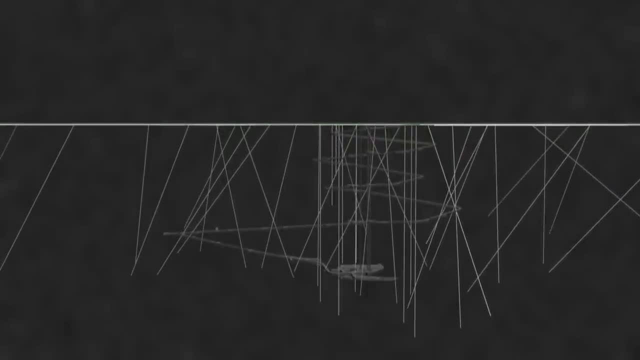 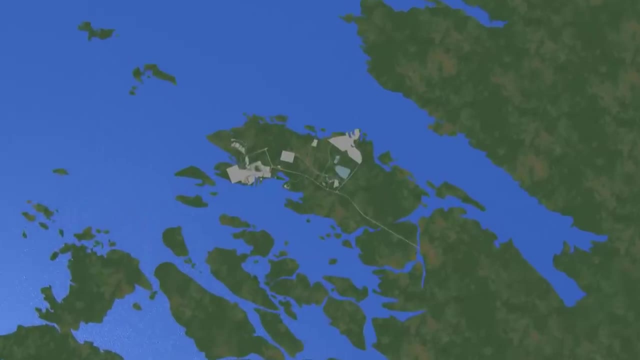 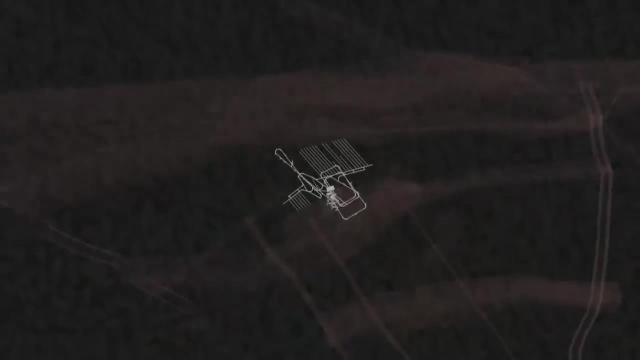 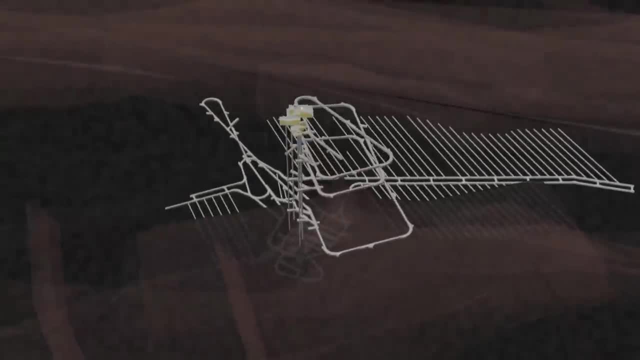 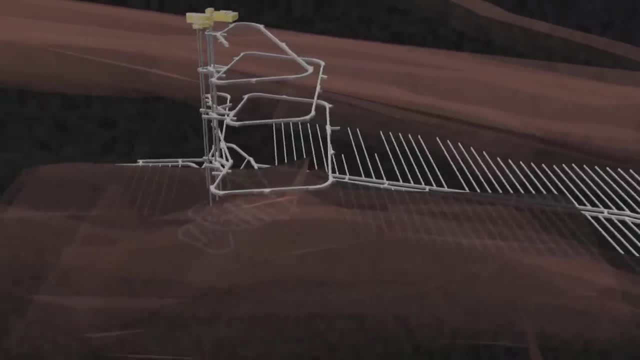 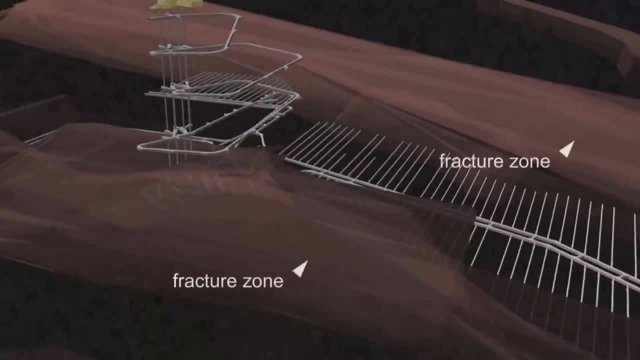 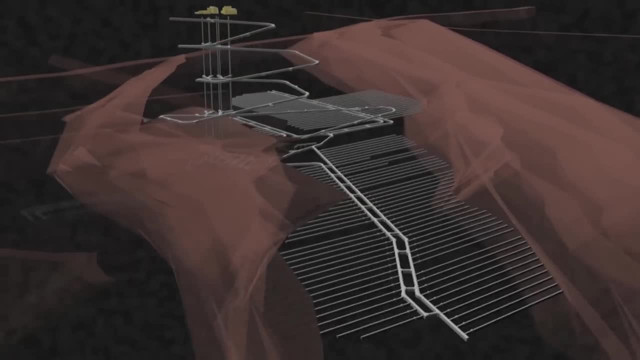 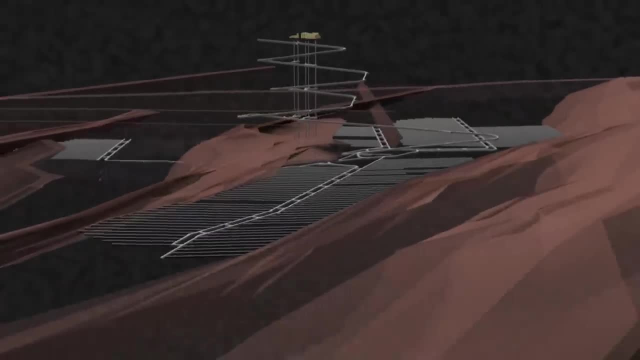 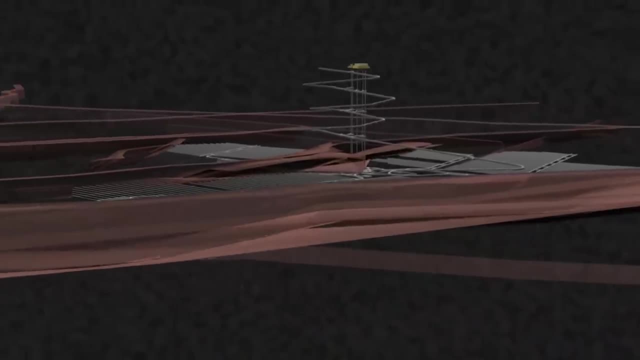 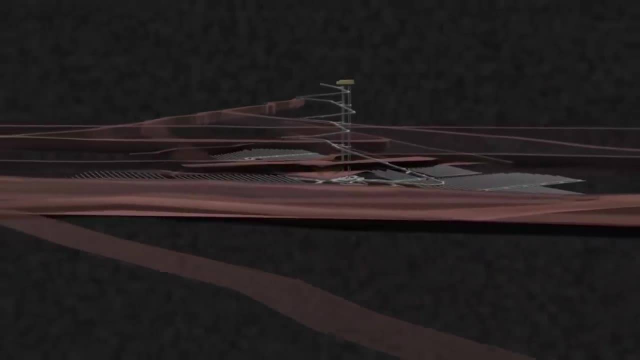 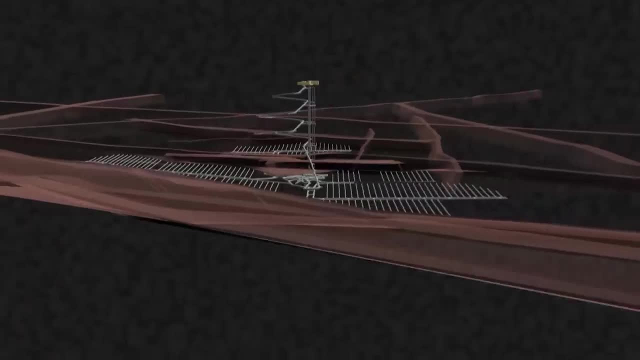 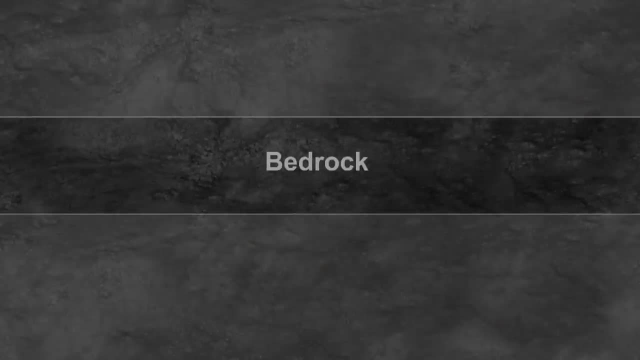 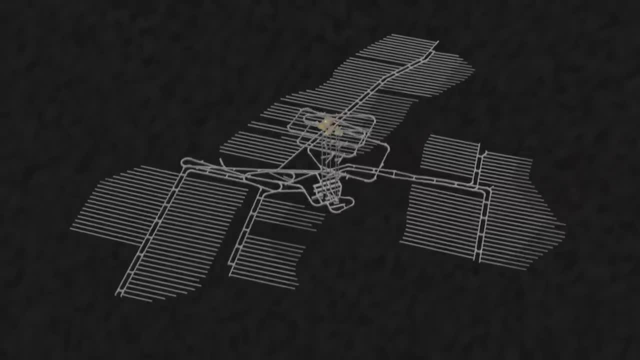 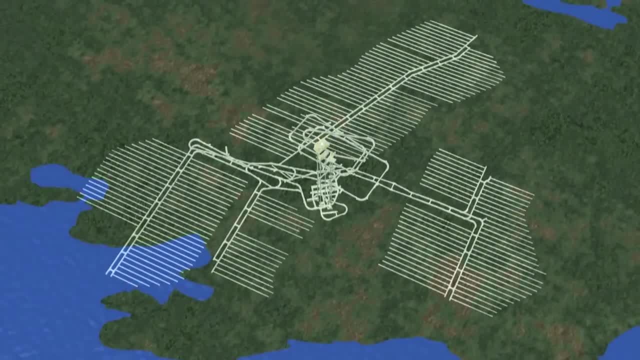 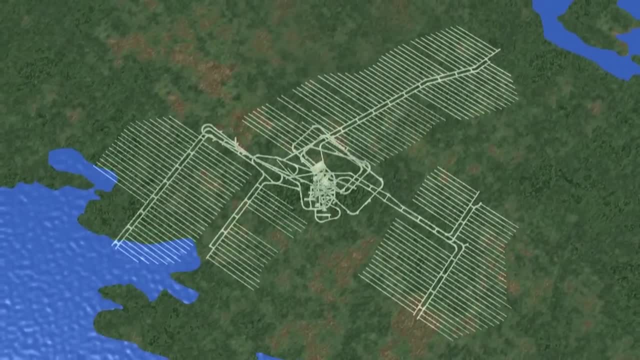 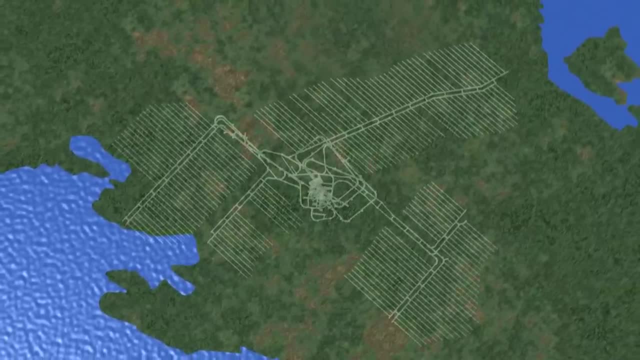 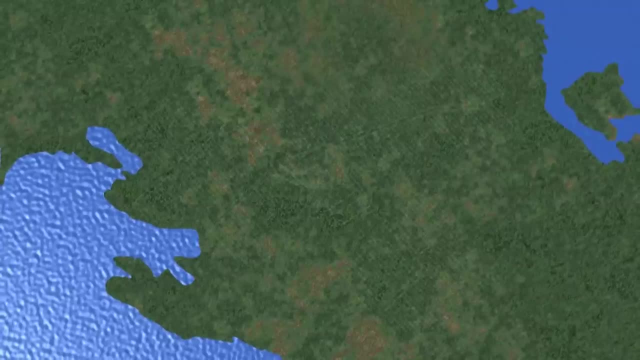 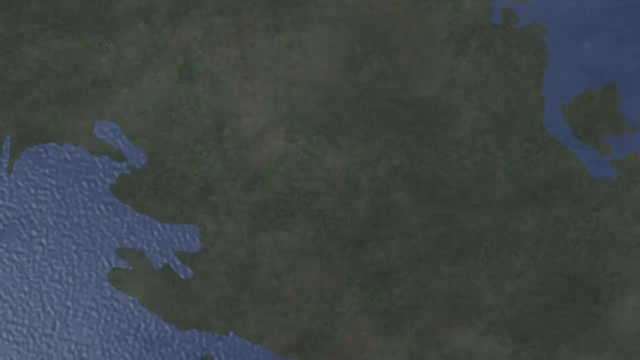 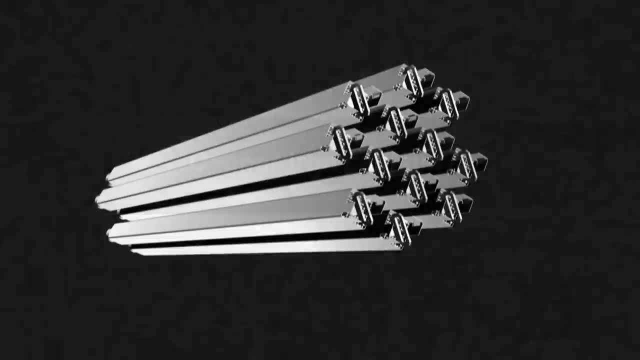 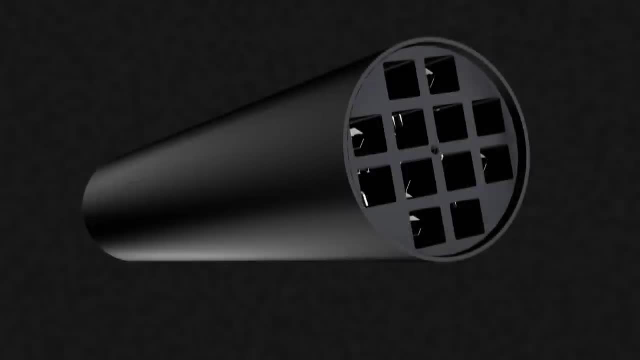 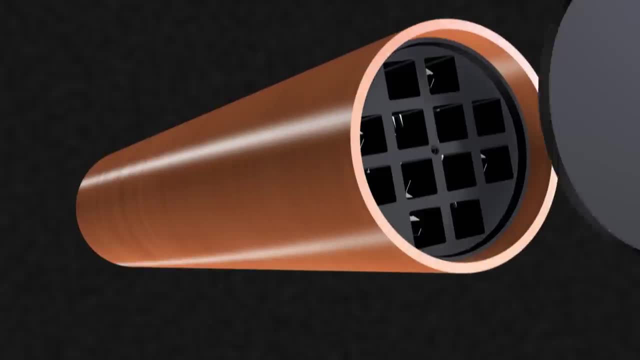 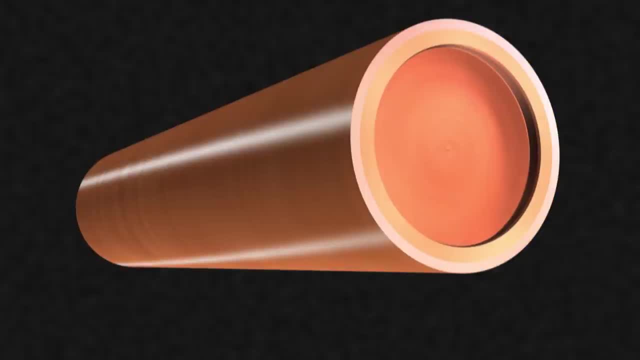 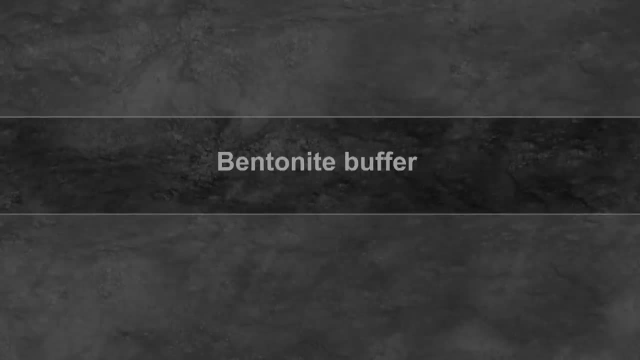 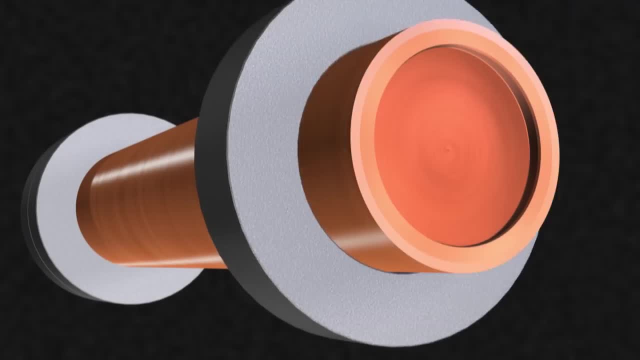 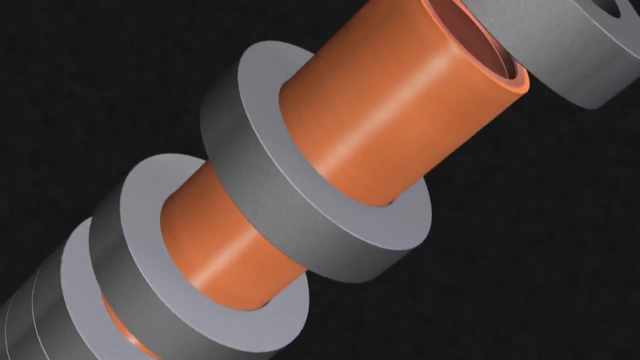 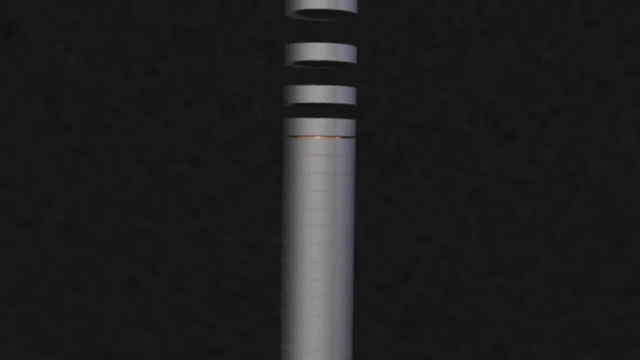 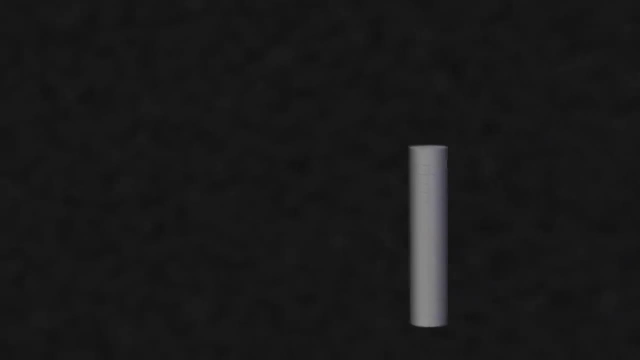 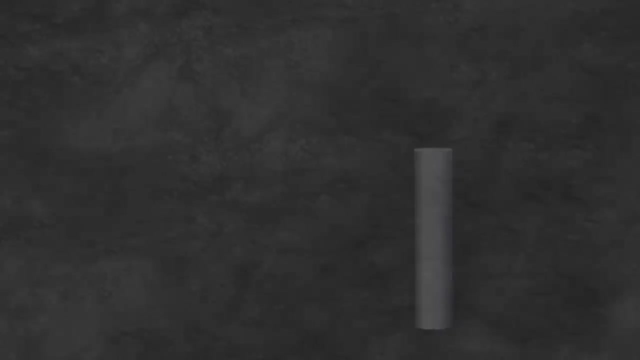 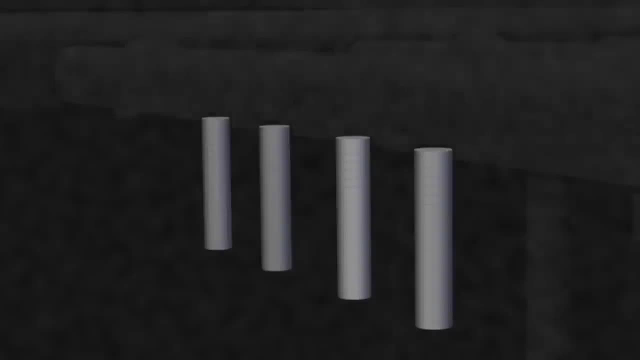 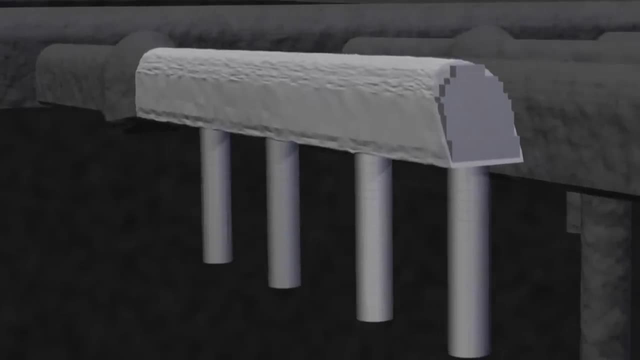 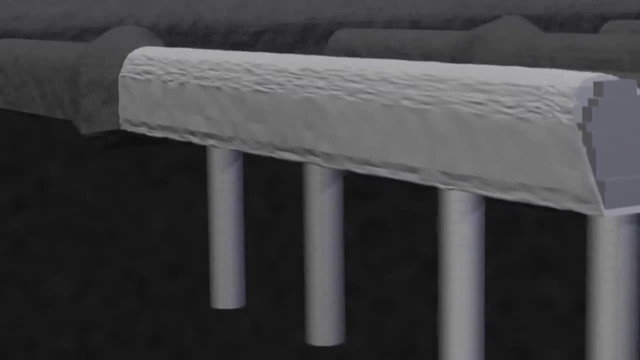 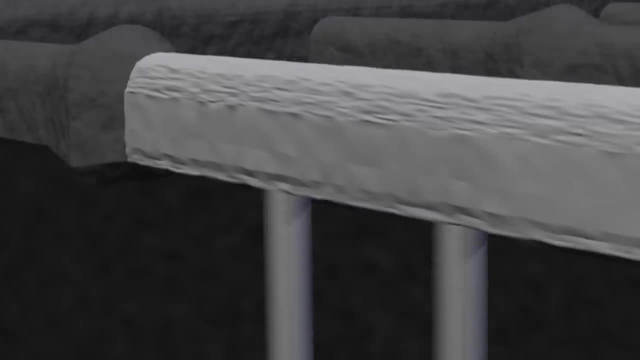 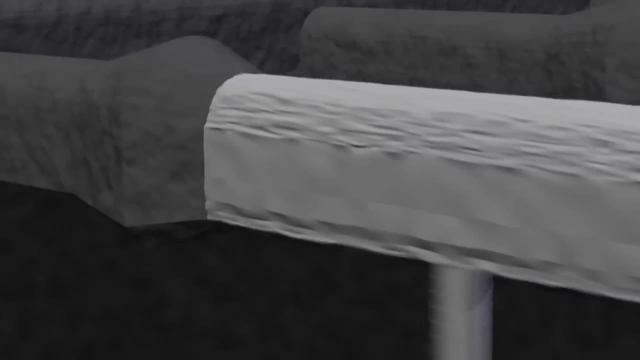 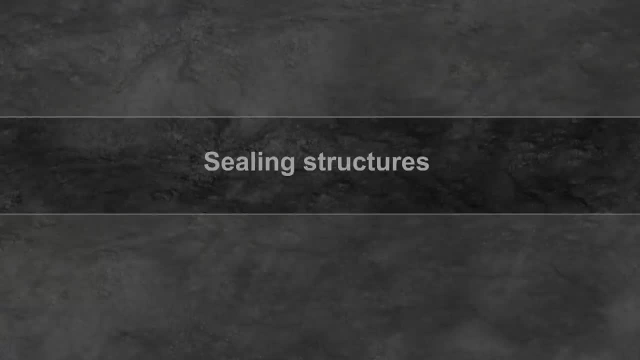 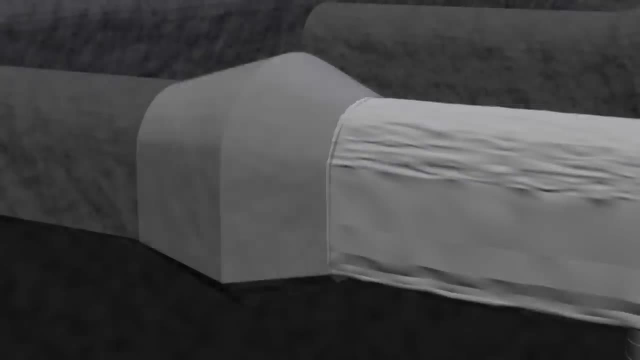 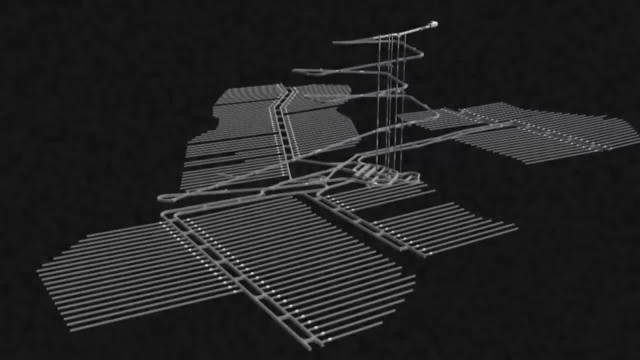 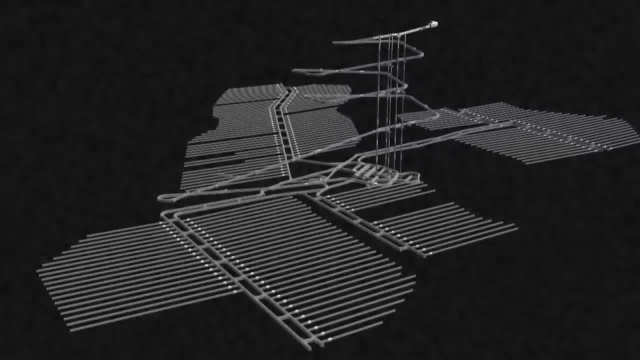 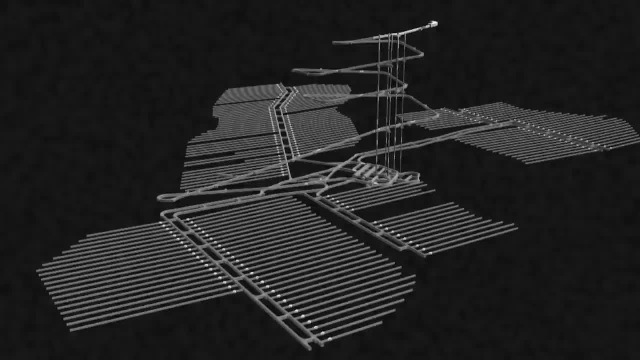 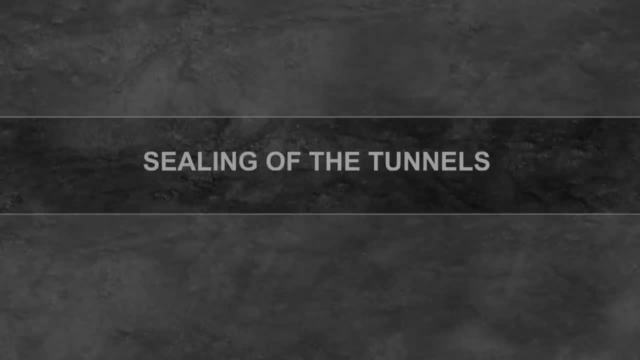 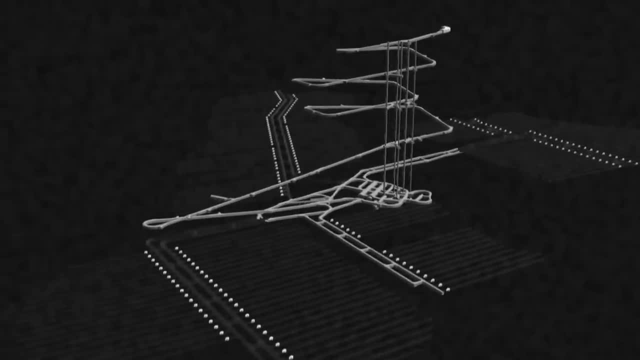 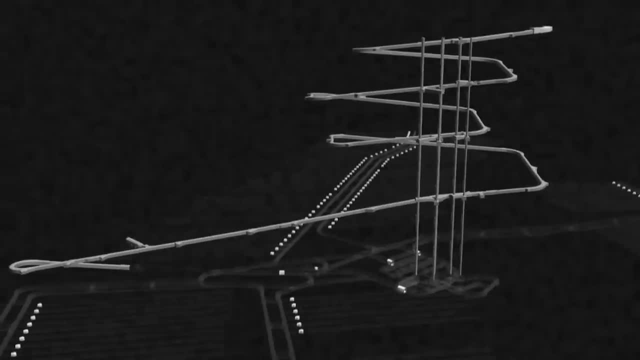 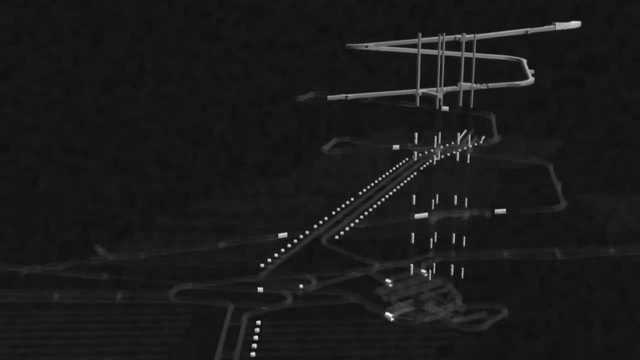 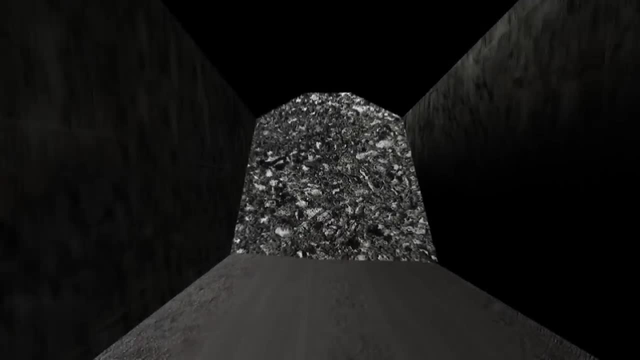 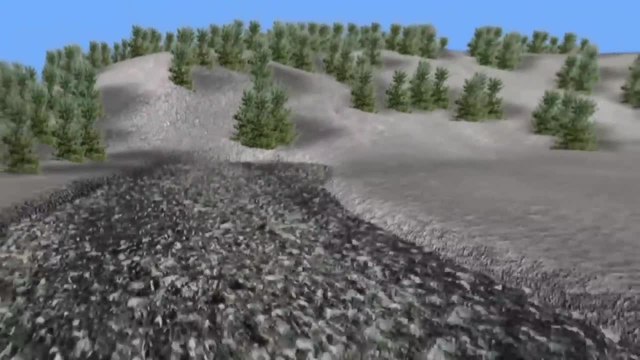 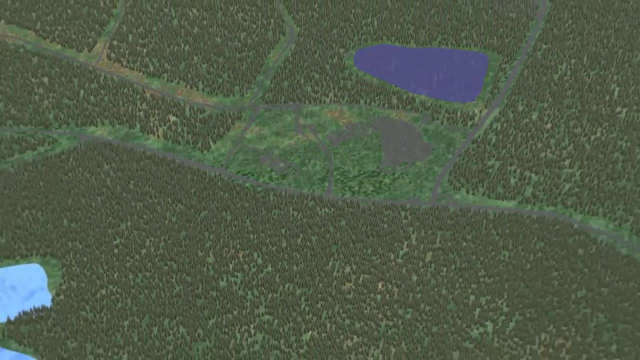 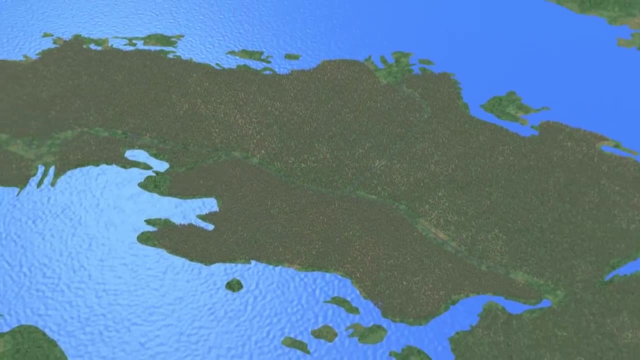 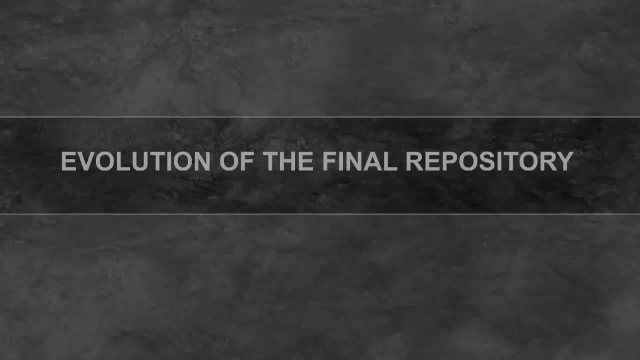 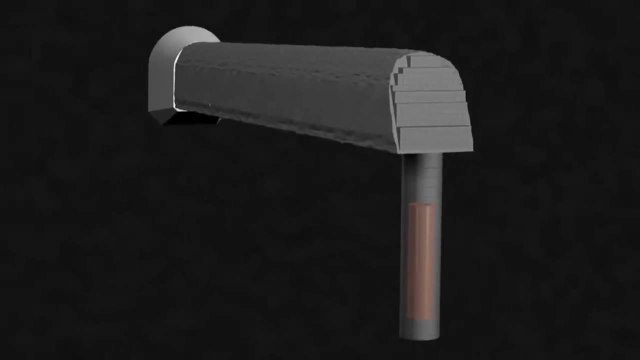 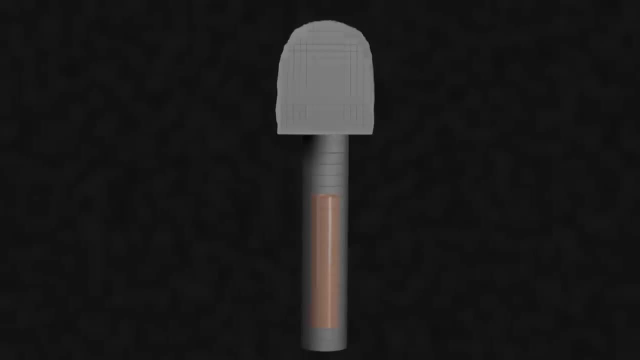 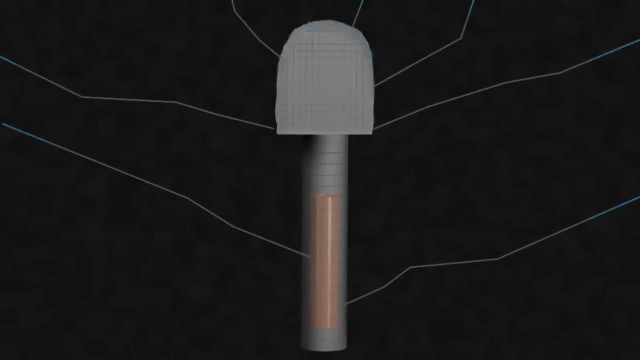 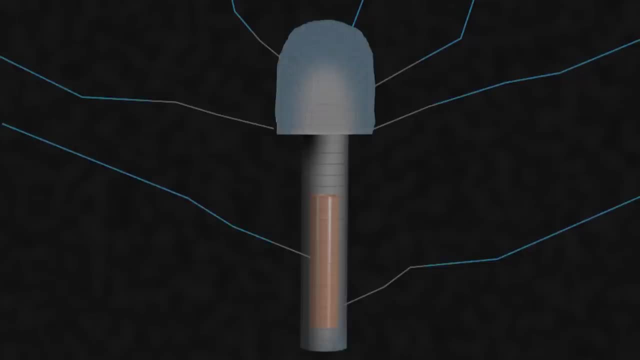 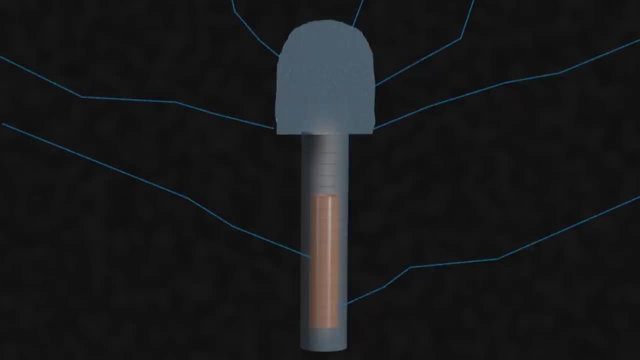 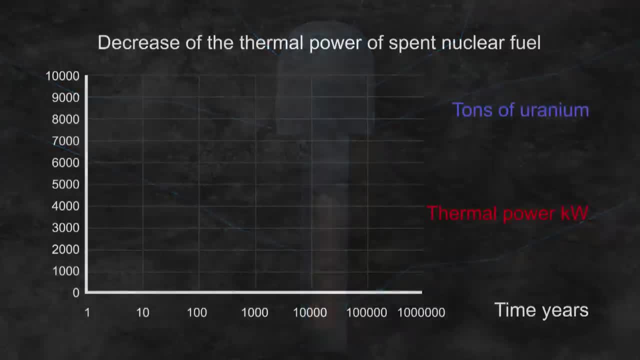 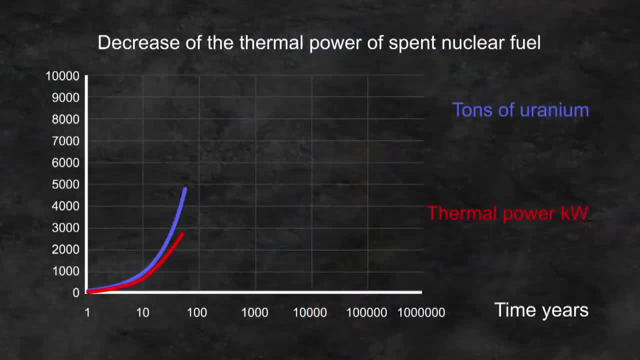 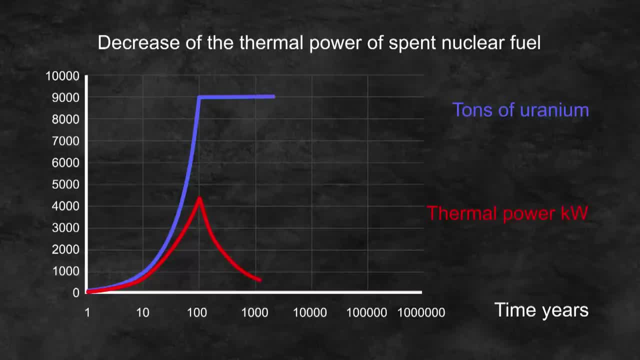 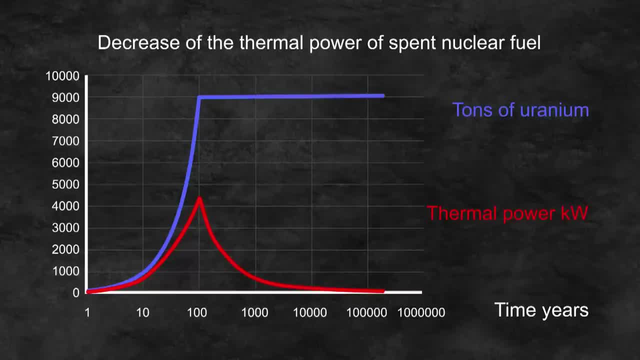 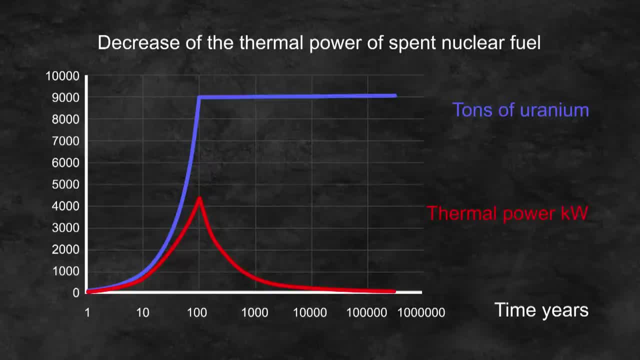 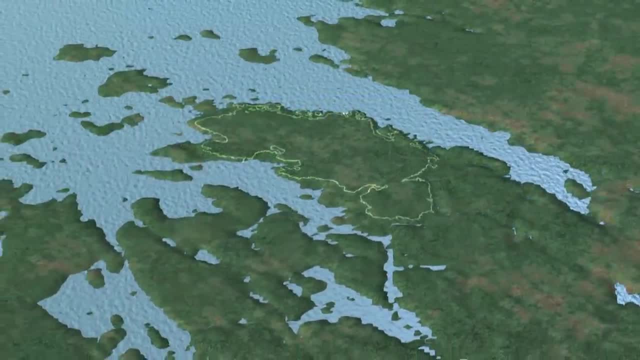 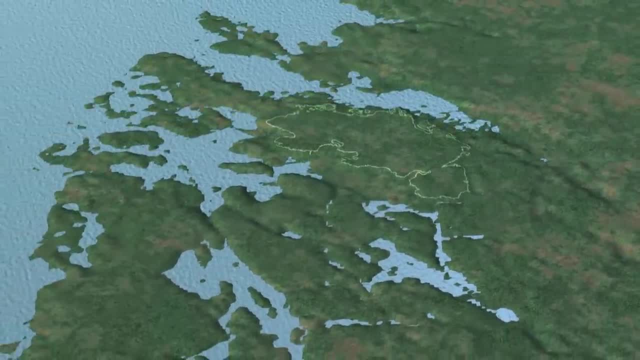 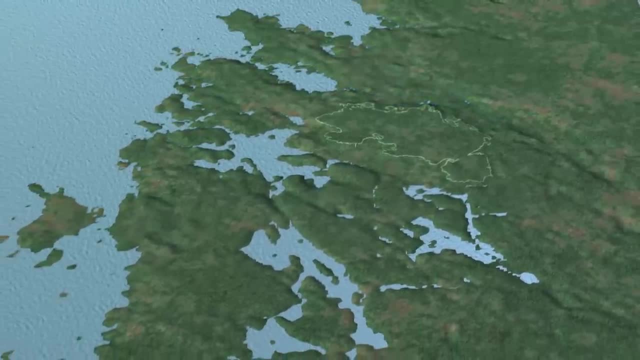 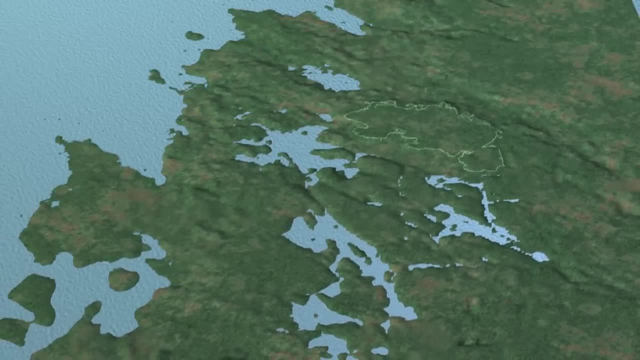 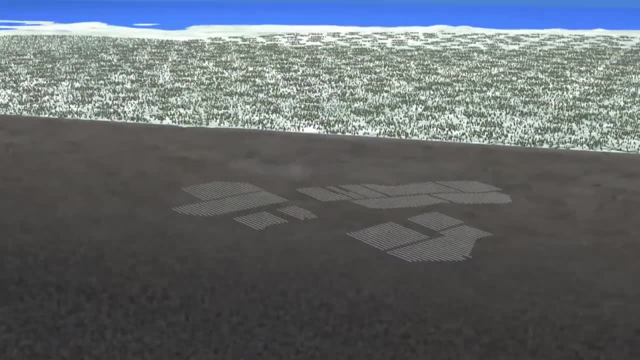 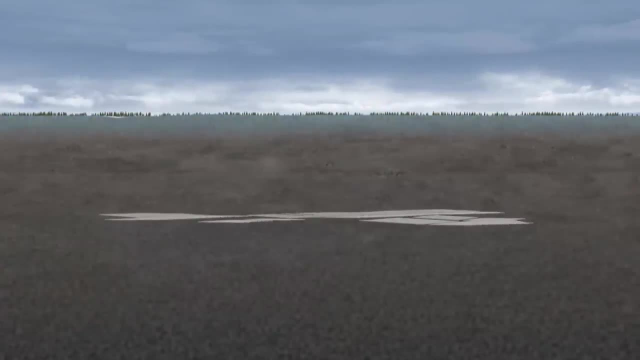 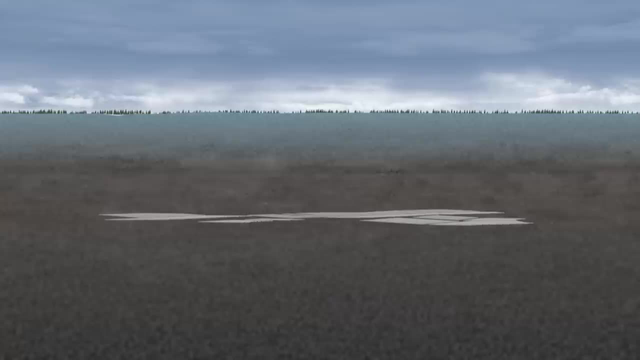 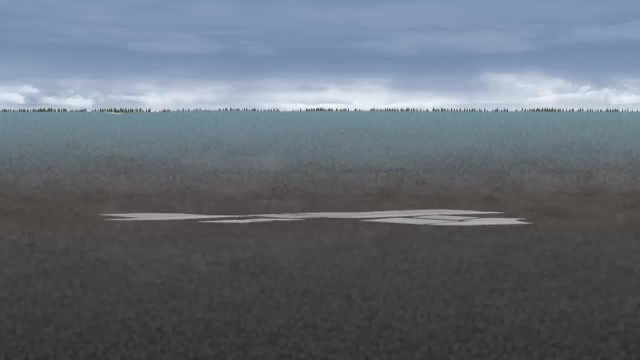 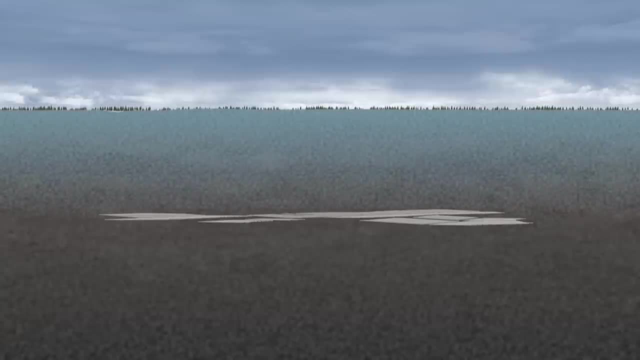 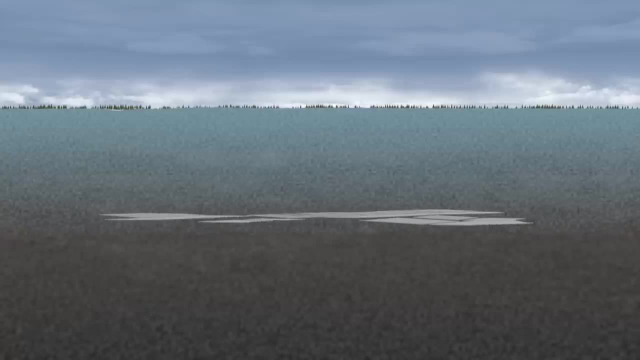 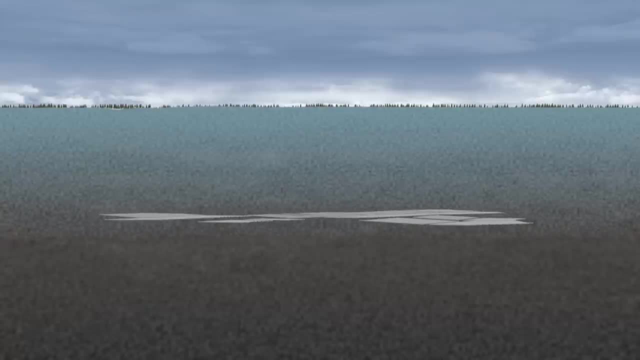 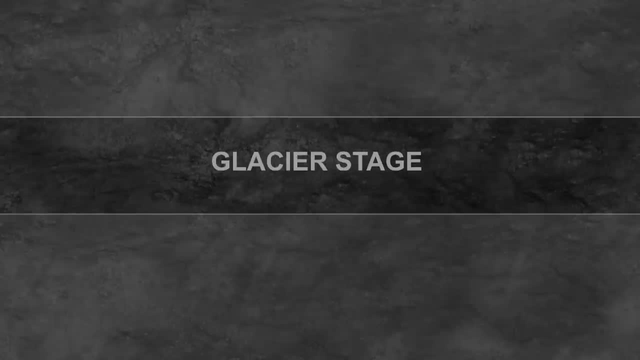 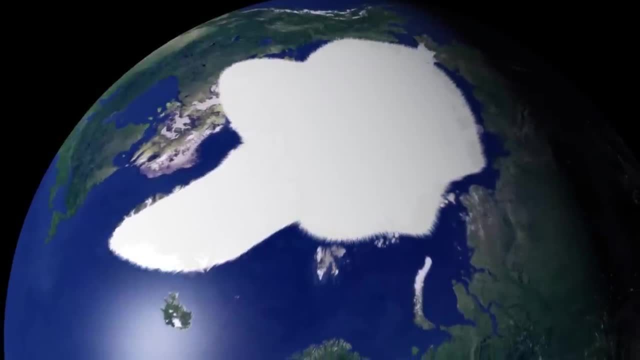 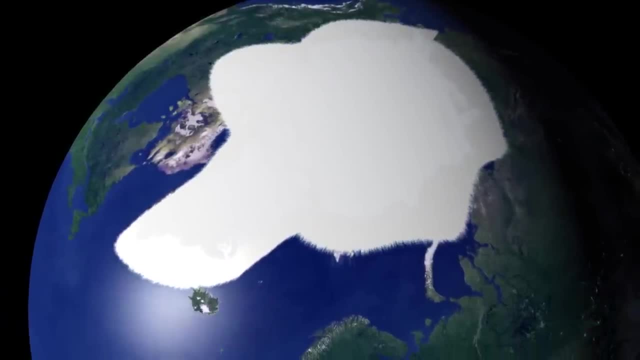 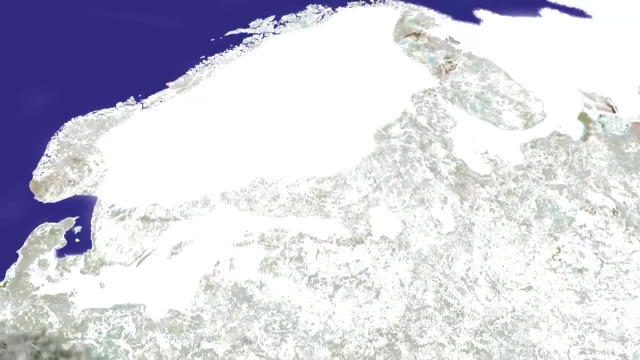 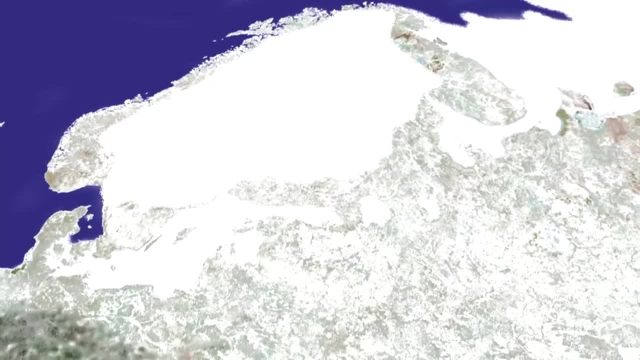 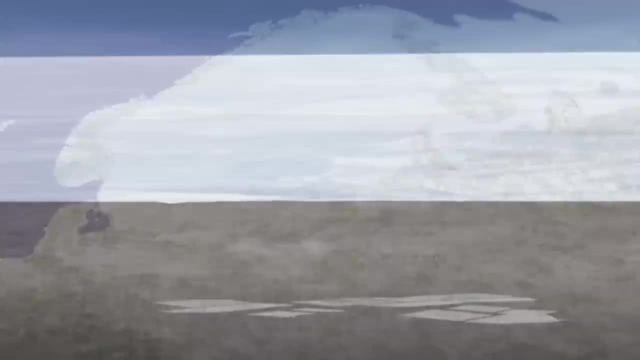 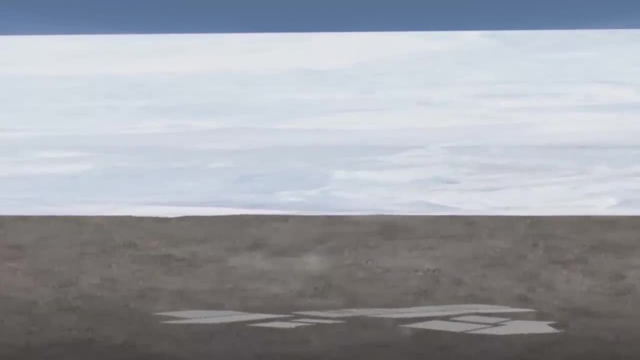 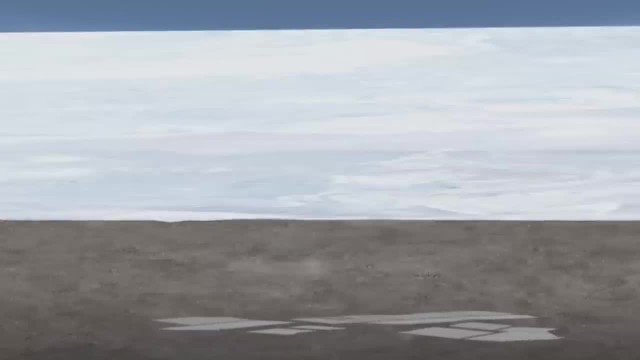 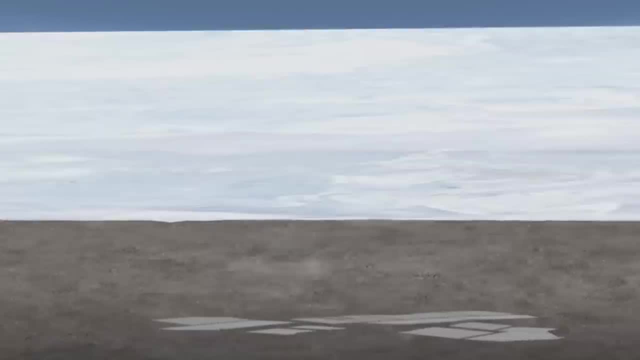 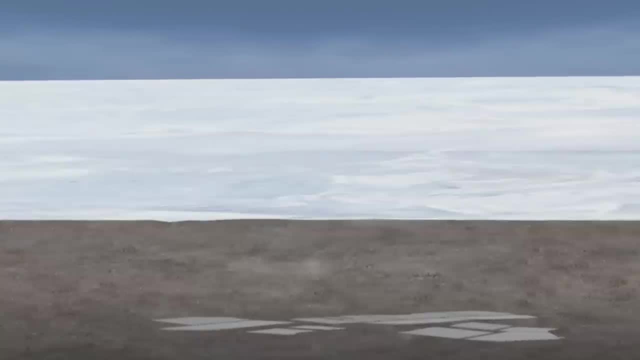 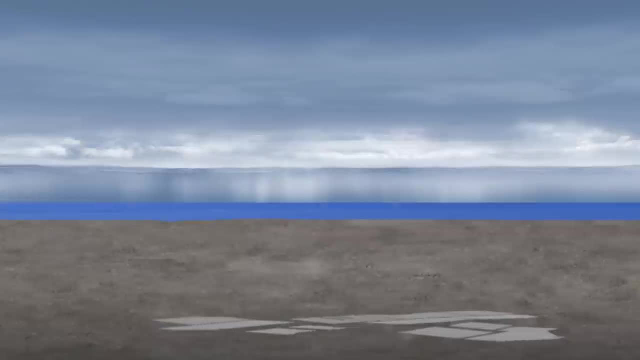 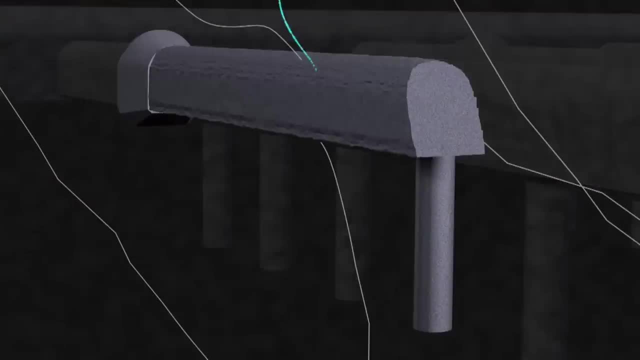 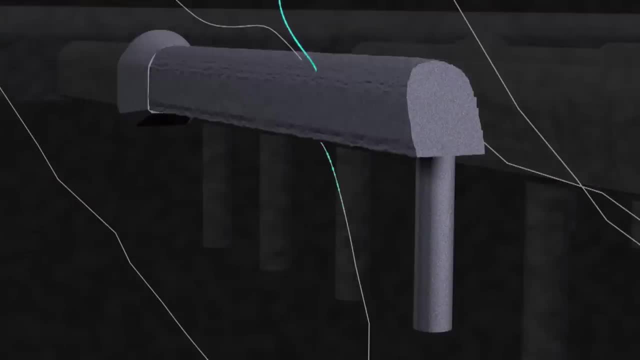 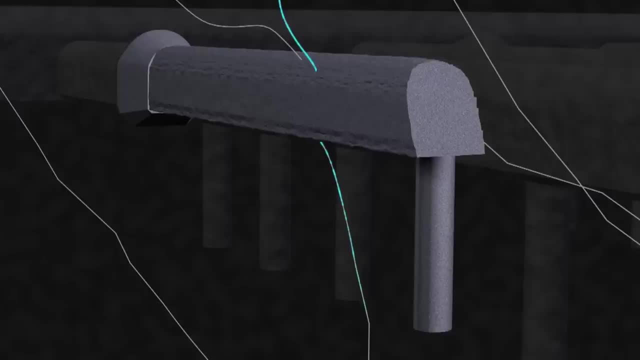 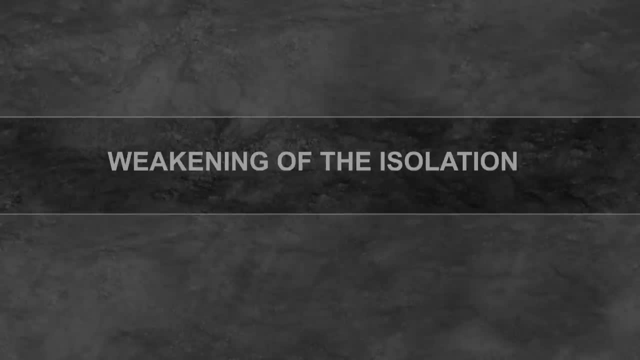 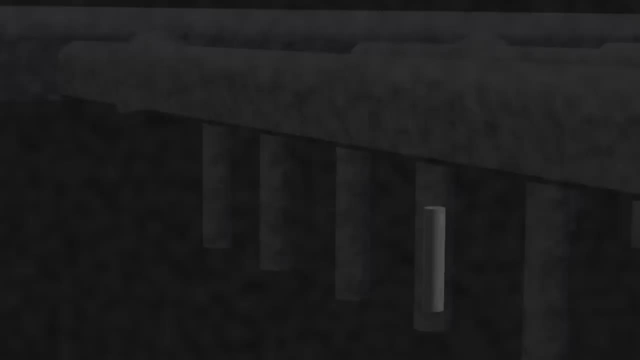 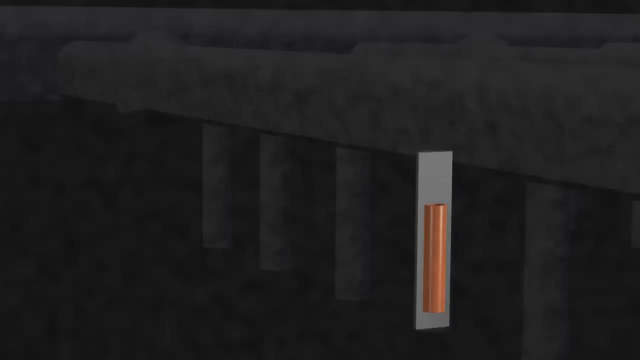 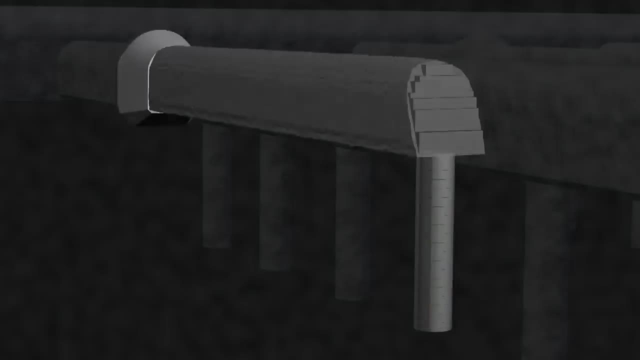 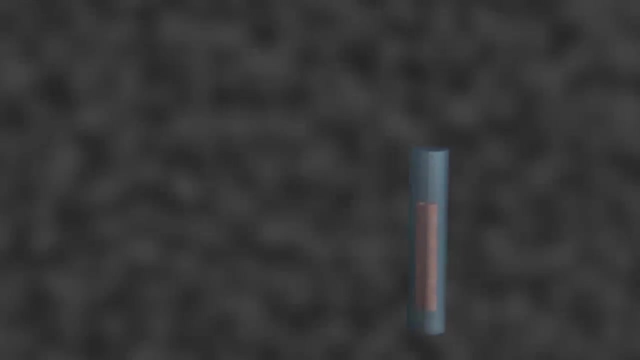 The animation provides the information about the basis for the launch of the facility. The animation provides the information about the basis for the launch of the facility. Therefore, unlikely scenarios are also considered when assessing safety. In such scenarios, one or more canisters lose their integrity.